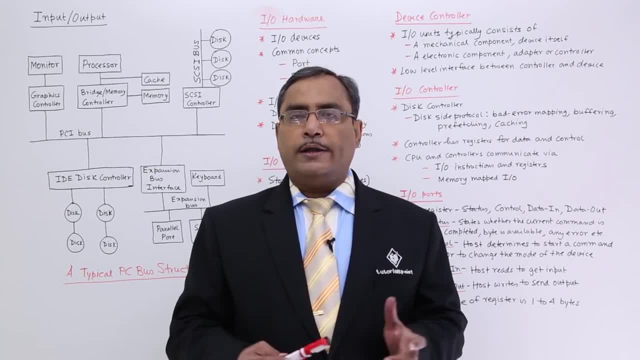 Topic for this session is input, output or I O. We are having multiple different types of input and output devices are getting connected with the main processor, with the main system. This input output devices mainly divided into two categories: One is a character oriented device, another one is a block oriented device. In case of character oriented device, the device- 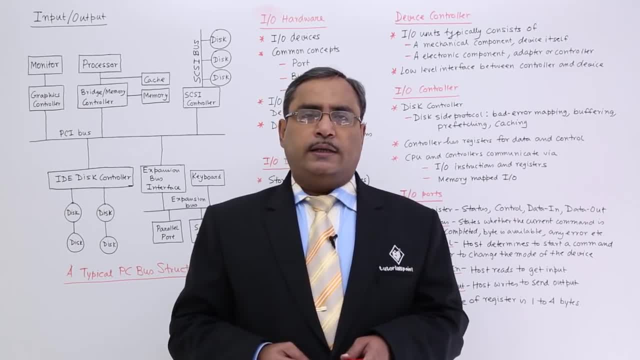 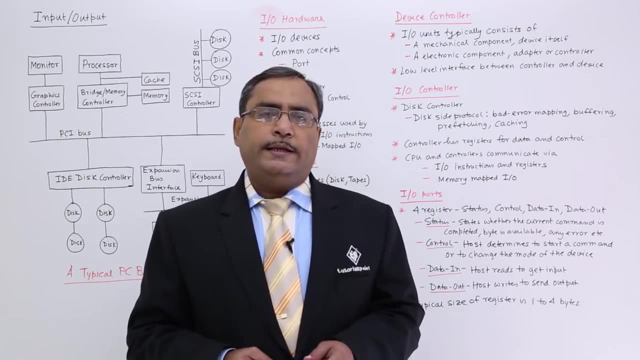 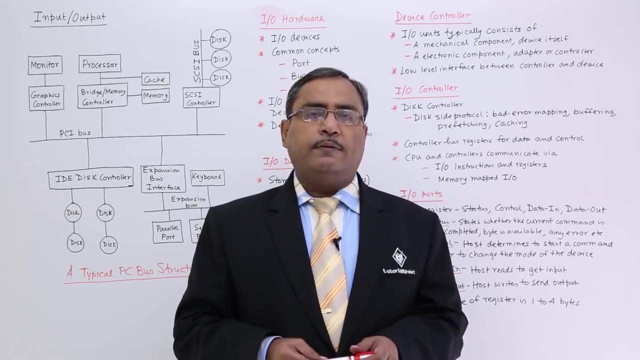 is byte communicable. That means a single byte can be transferred, can be read, can be sent in between the device and the system. In case of block devices, that device will do the communication with the chunk of data in the form of a block: Mouse, printers, keyboards. 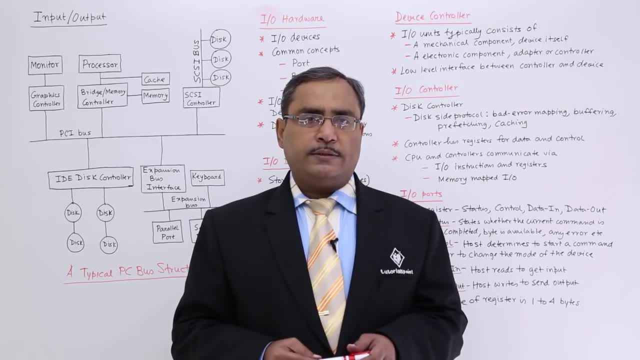 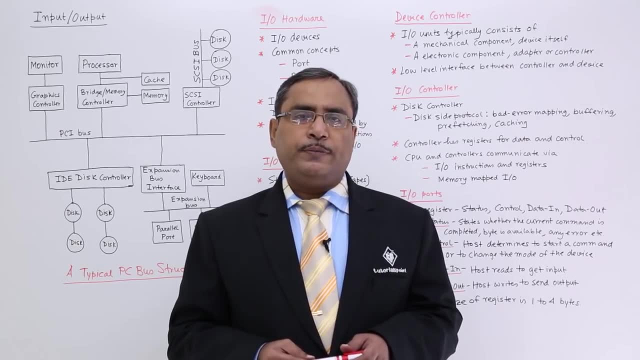 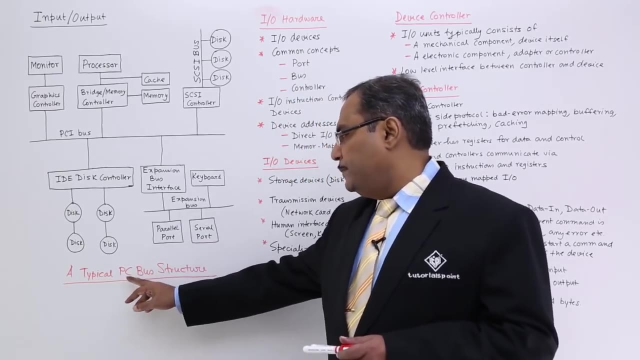 are the good example of byte communicable device or character oriented device, and all the disks should be connected. So to have a detailed discussion on this particular I O, I have drawn one block diagram, a typical PC bus structure. So here I have tried to show you that, how the different devices 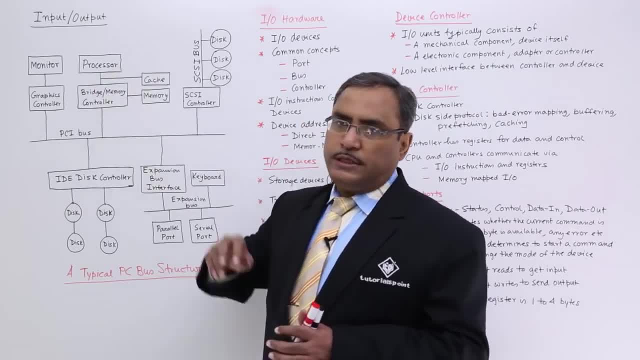 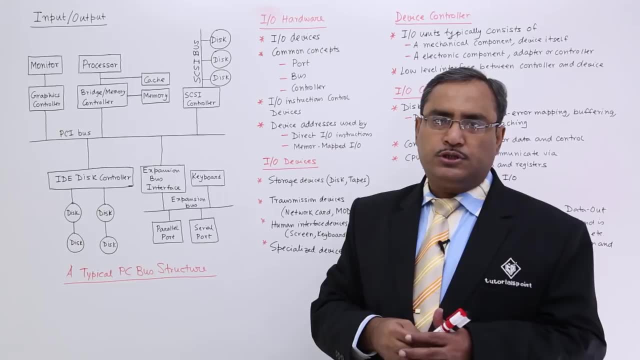 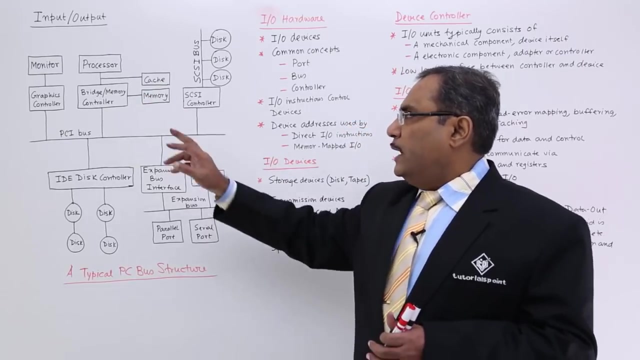 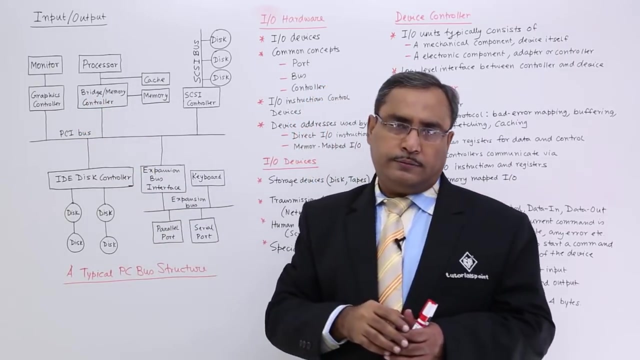 are getting connected. Now, this is my main processor, the CPU, and this processor is having the cache memory connected, obviously because processor will store its required and frequently required data or instruction in this particular cache memory. And with this particular main memory it will be having one control unit and that is the bridge memory controller. 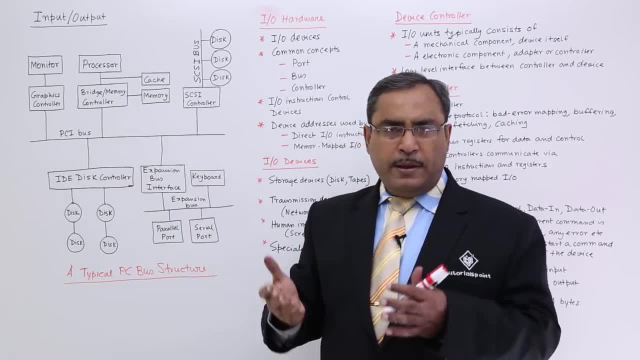 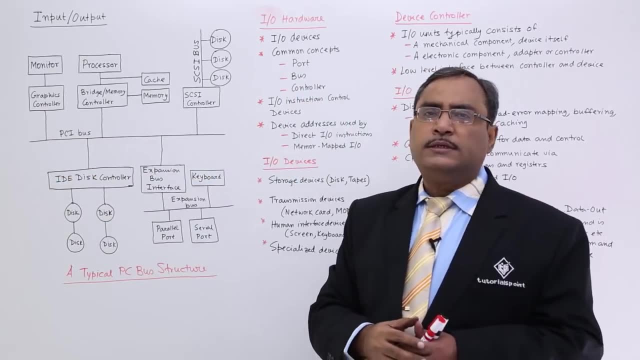 And this particular data which will be coming to the memory may be coming from some I O devices, So that is why it is known as the PCI bus or it is also known as I O bus. The full form of PCI is peripheral component interconnect. This PCI bus can be connected to the PCI bus. 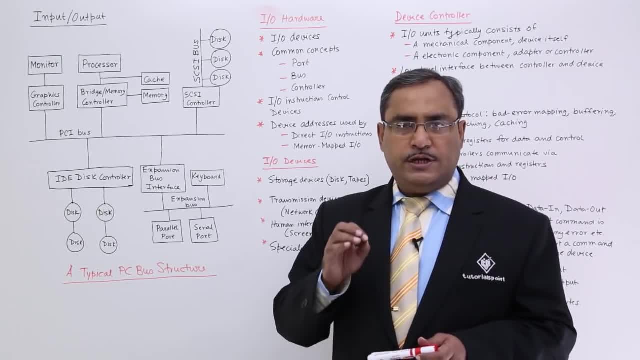 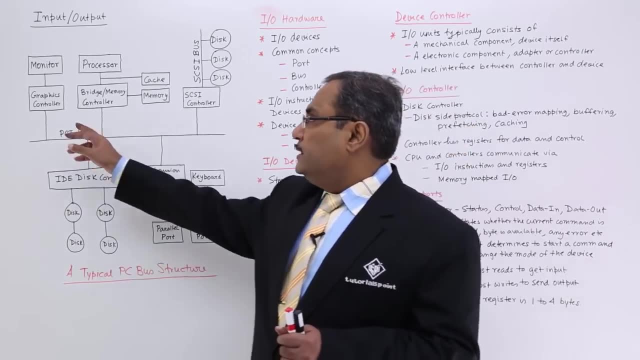 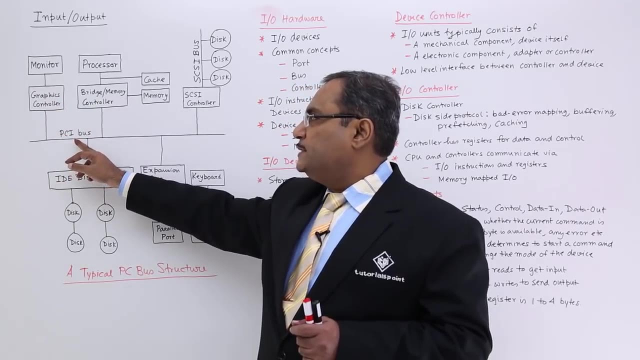 PCI bus can also be called as the I O bus, because it is dedicated to have or to establish a communication between the system and the I O devices. This is my monitor, on which the display will take place, So it is getting connected with the PCI bus through a controller. 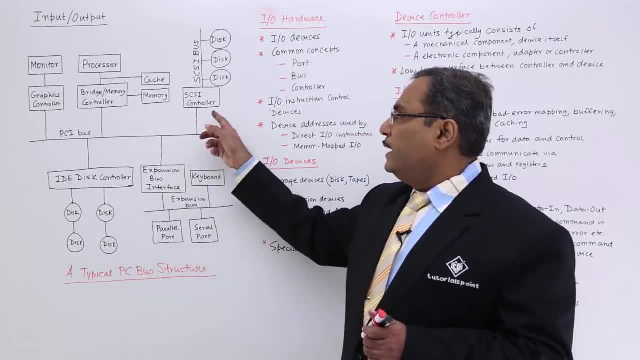 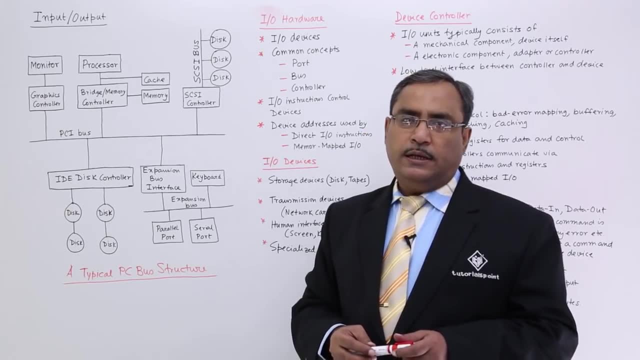 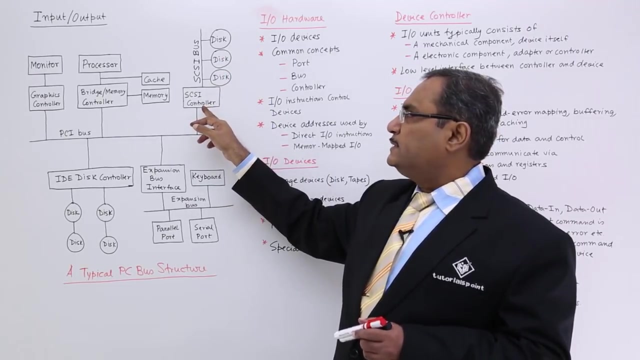 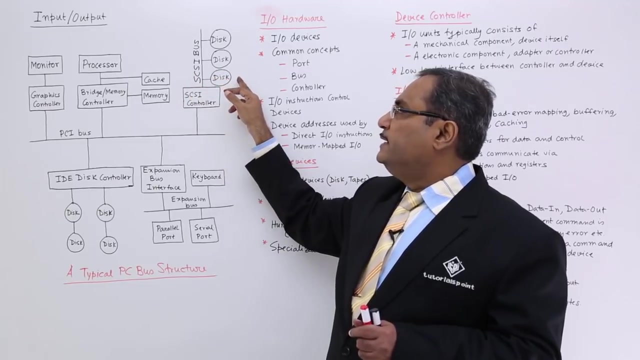 known as the display or graphics controller. Here we are having the SCSI controller. The full form of SCSI is small computer system interface And with this particular SCSI controller high speed hard disks are connected. So this particular SCSI controller will provide SCSI bus And with this SCSI bus these disks will remain. 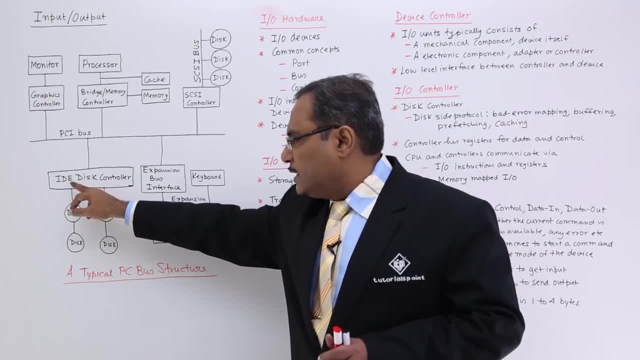 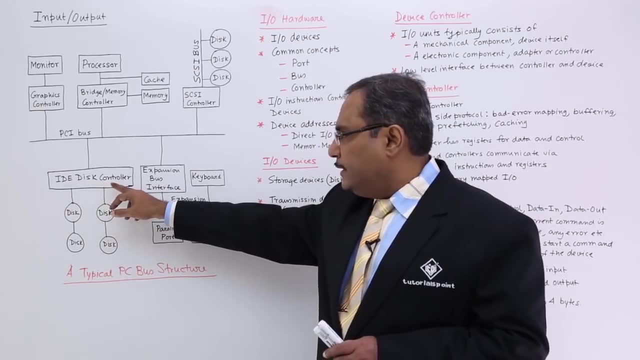 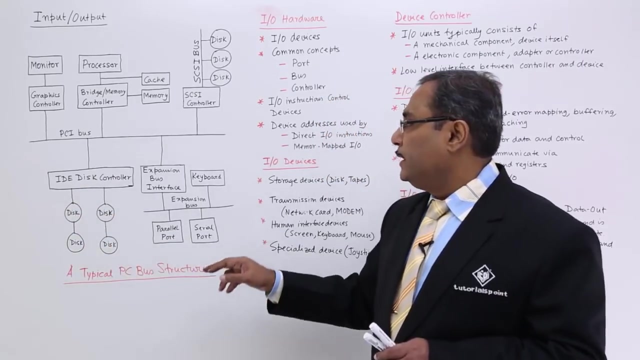 connected. We are having another kind of disks, So that is the IDE disk controller, integrated device electronics. So with this particular IDE disk controller we are having multiple number of disks connected With the local dedicated disk buses. So now here we are having this expansion bus interface. 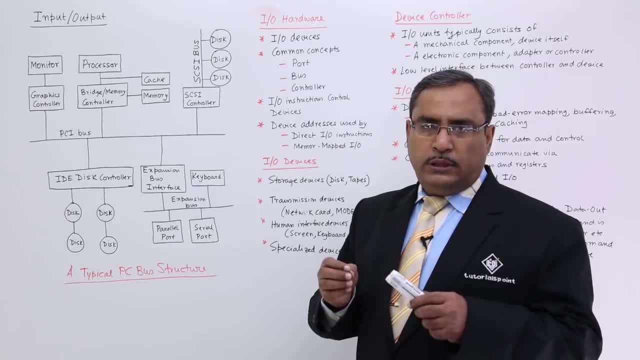 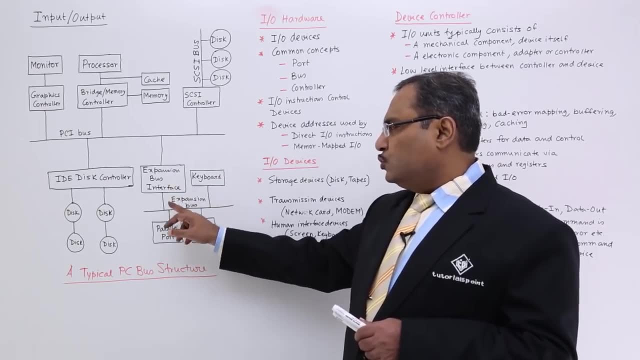 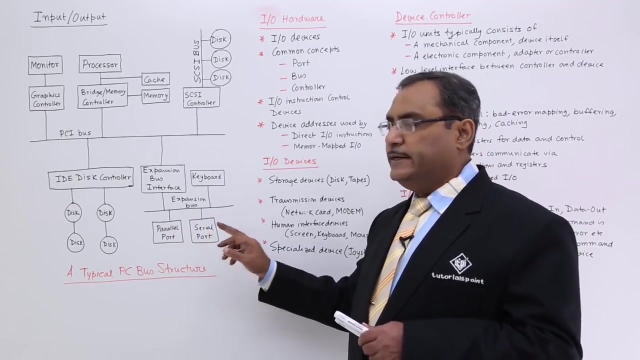 So where we can have more ports and with the help of the ports we can connect other peripheral devices. So like keyboard, it has got connected. This. ports can be mainly categorize. ports can be categorize in two different heads. One is the parallel port, another one is a. 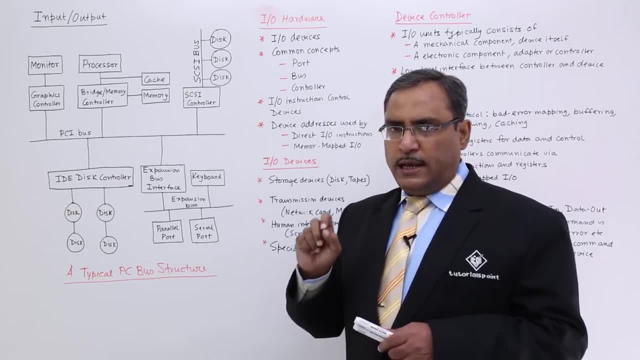 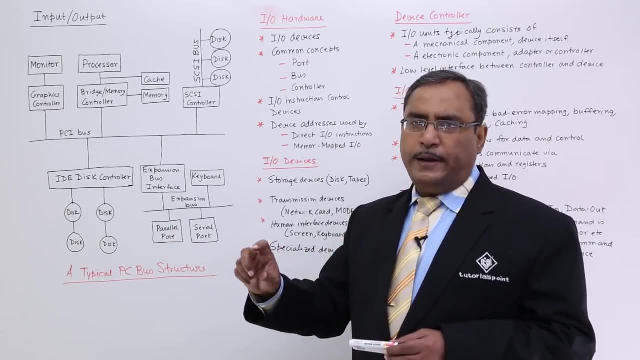 serial port. In case of serial port, against each and every clock pulse, I shall be getting bit at a time for the communication. In case of parallel port, we will be having multiple number of bits. mainly one byte of information can be transferred against a single clock. 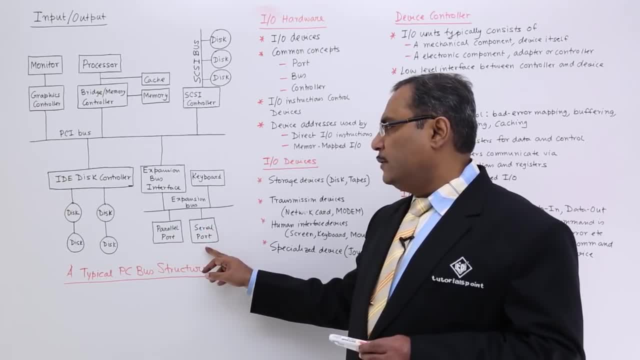 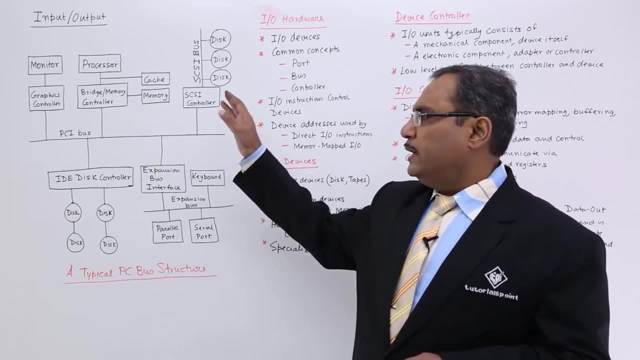 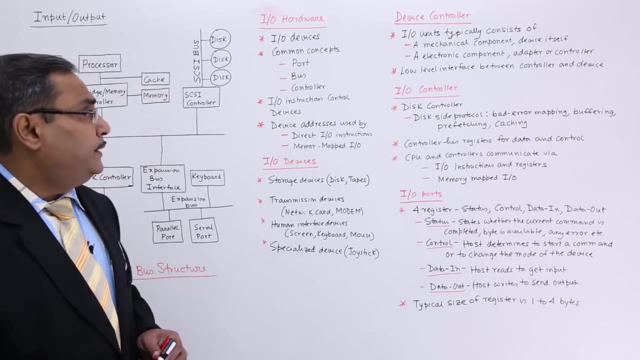 pulse. So this is the parallel port and this is the serial port. Expression buses are there, with the help of which you can connect other peripheral devices. So in this way, we have discussed this particular typical bus structure of a PC. Now see in case of I O connections. 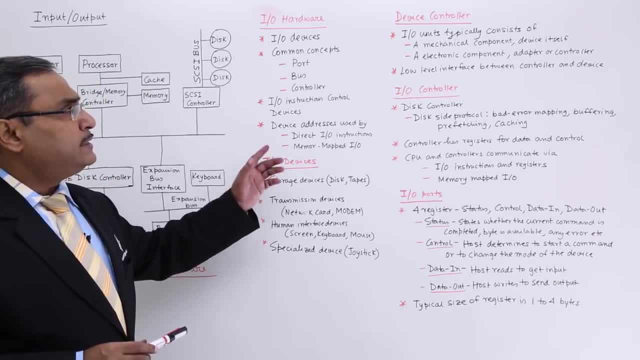 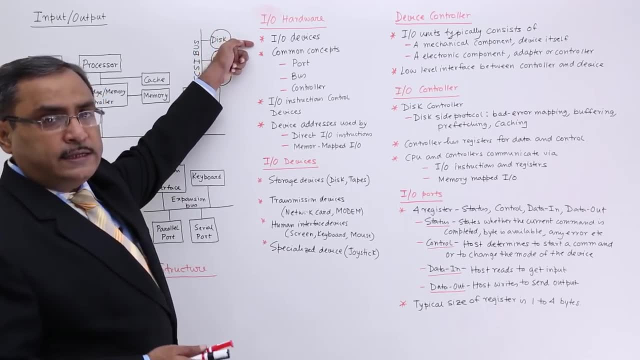 we are having some I O hardware, we are having some I O devices and so on. So I O hardware is mainly having this components. So one is the I O devices. obviously it will be having different I O devices that will be the part of the I O hardware And there are some common. 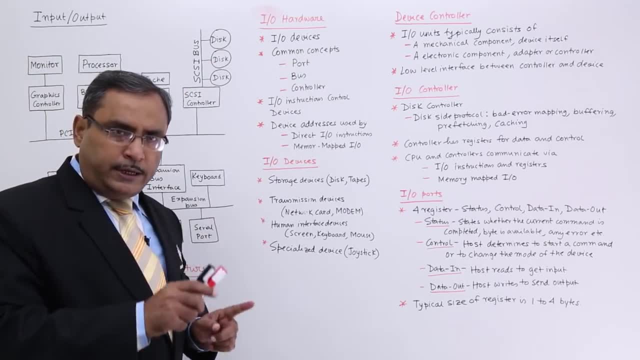 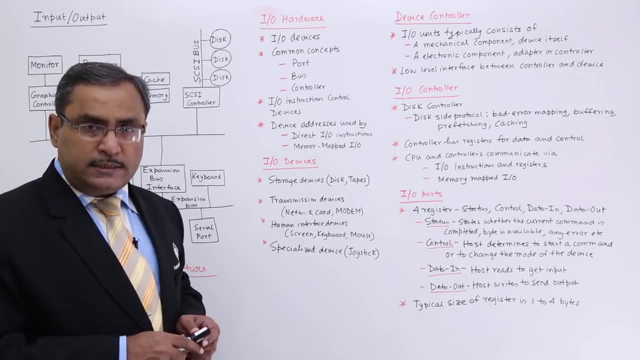 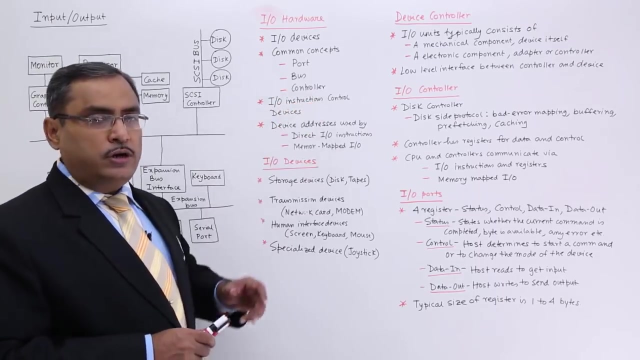 concepts like port, Where the system will get connected with the peripheral device, A common interfacing point that is known as a port. We are having different kinds of buses- We know that we have here shown that- the PCI bus and other SCSI bus and so on- And we are having controllers. 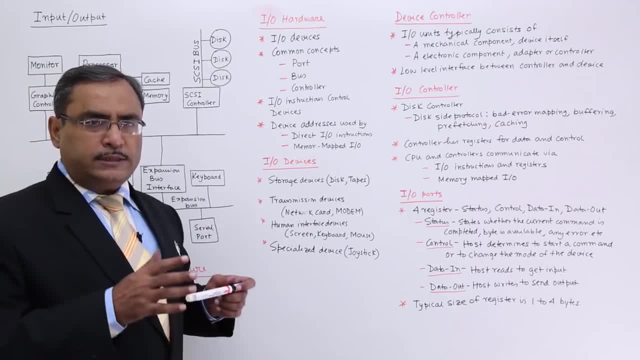 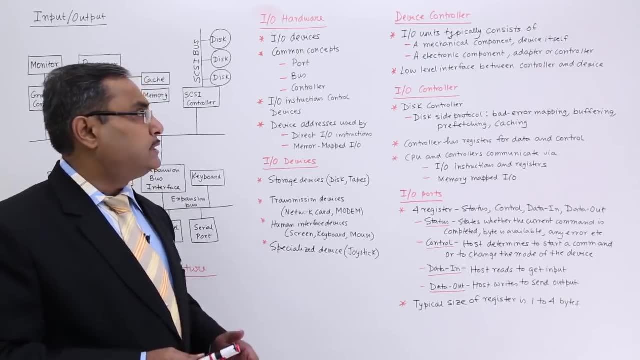 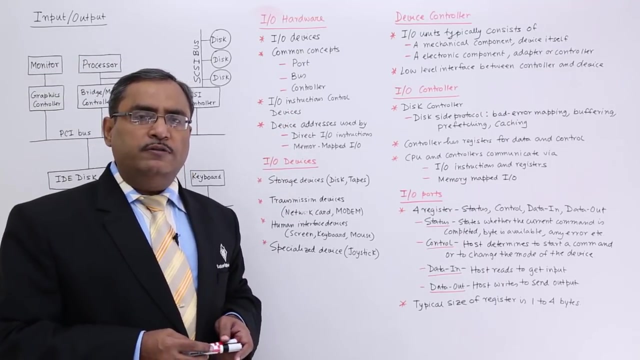 With the help of controllers we can do the communication between the system and the buses. The controller will produce different control signals to decide what will be the usage of the bus. This bus can be can have contention. that means more than one i o devices may be demanding this particular bus. 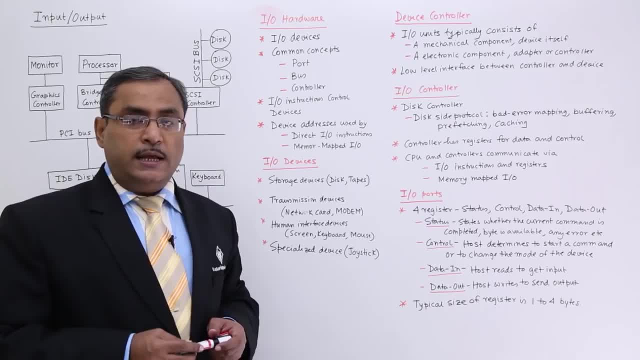 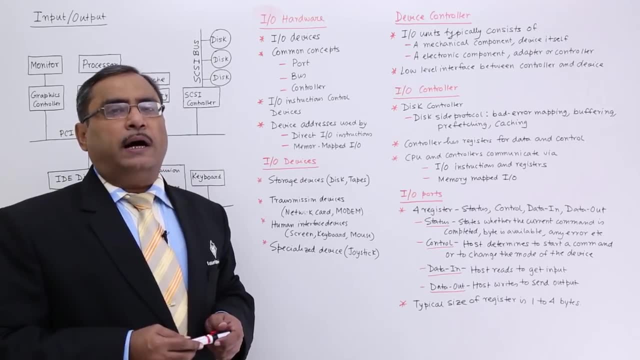 so that is why this bus contention may take place, and this bus contention will be resolved by a technique known as bus arbitration. this bus arbitration will be controlled by bus controller or bus arbitrar. there are three different methods with the help of which this bus arbitration can. 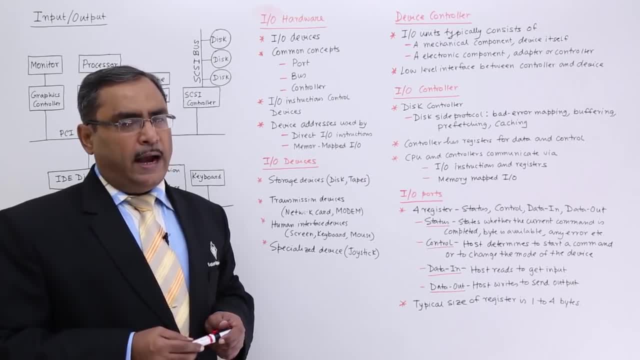 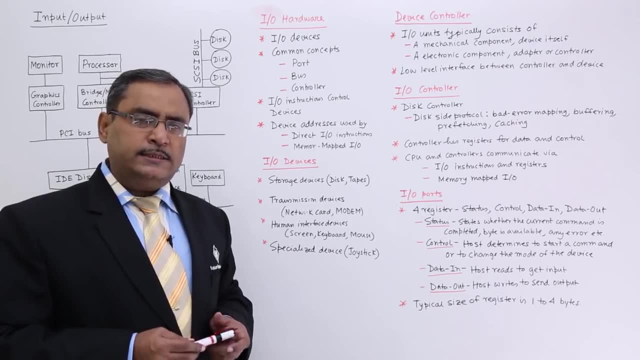 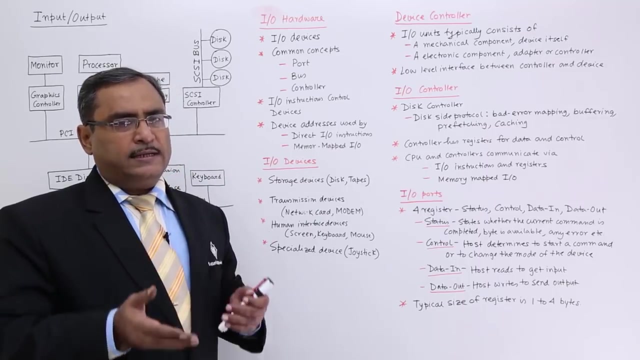 be done. one is the desi- sue arbitration, another one is the polling, another one is the independent requesting desi. changing arbitration means in this case the module wise will get the permission at a time. the first module will get the permission to do or to access the buses. if the module is ready to access the bus, it will access it. otherwise the bus grant. 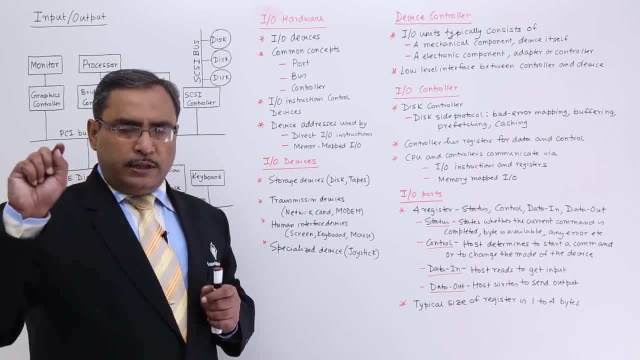 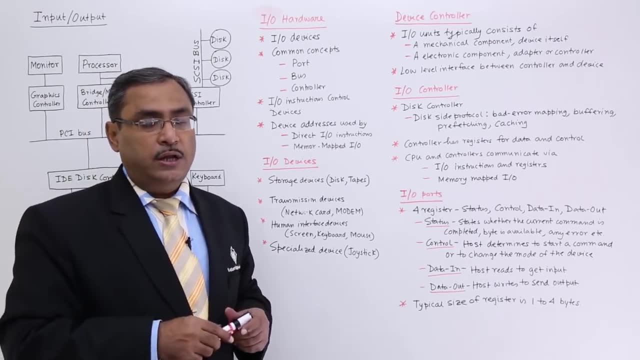 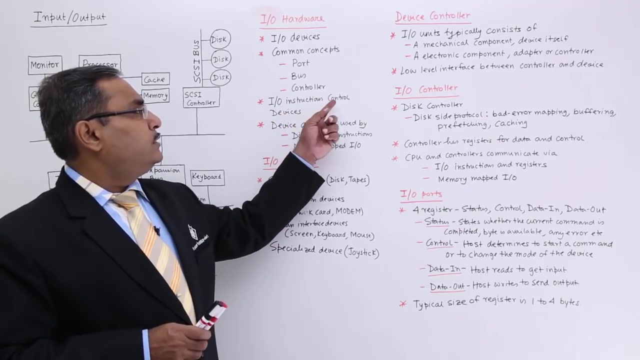 or this permission signal will be transferred to the next module. then it will be transferred to the next module. in this way it will proceed. So that is known as the daisy chaining arbitration. So other arbitration techniques are polling and independent requesting. So we are having IO instruction control devices. So there will be some device which device? 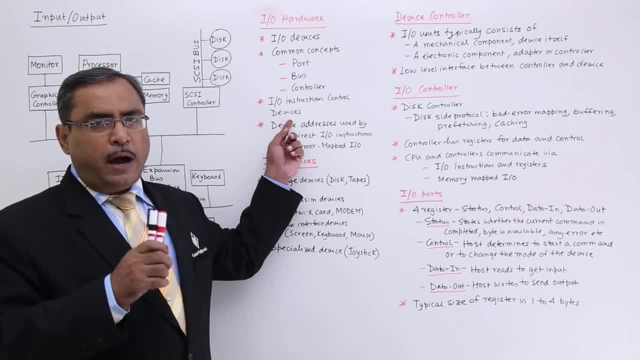 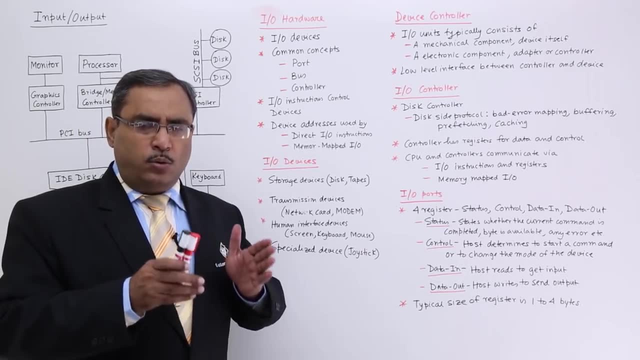 will do a communication between the CPU and the respective IO ports. So also they are known as programmable interfacing devices. So this particular devices will be having some ports connected and there are some control words with the help of which you can decide. 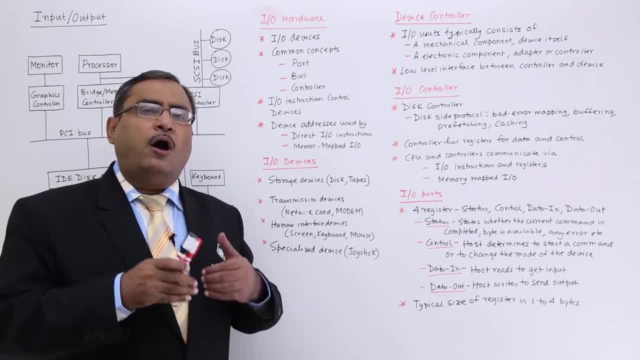 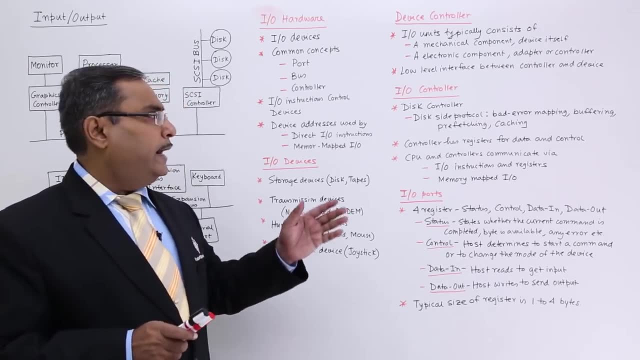 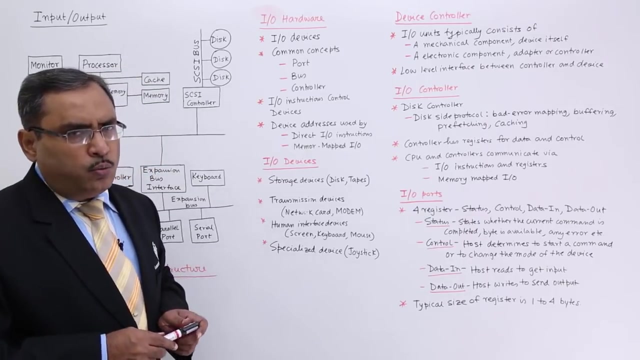 whether a port will be used as an input port or output port and whether what are the different control signals are to be initiated, and all these things will be guided by this IO instructions. control devices And device addresses can be two types. Actually, one IO device can get mapped with a system in two different ways. One is known as a direct. 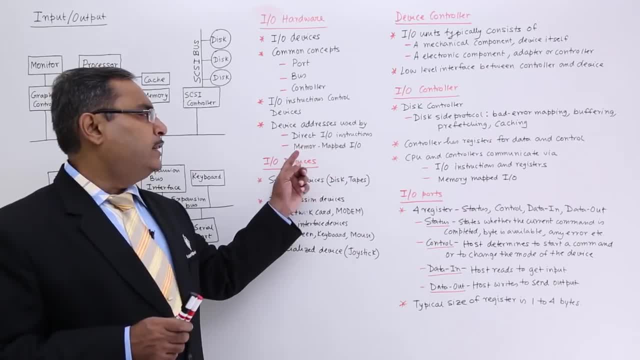 IO instruction control device. The other one is known as the direct IO instruction control device. The other one is known as IOMapped IO and another one is the memory mapped IO, So another one is the memory mapped IO. So what is the IOMapped IO and memory mapped? 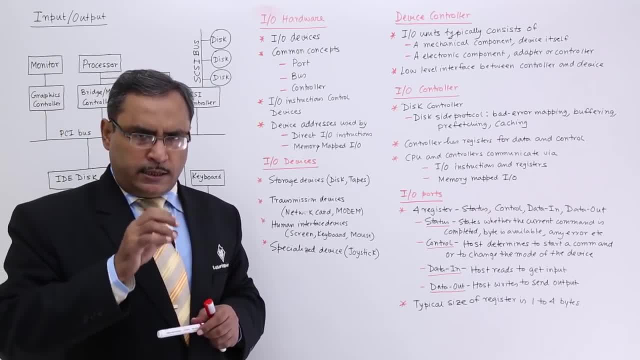 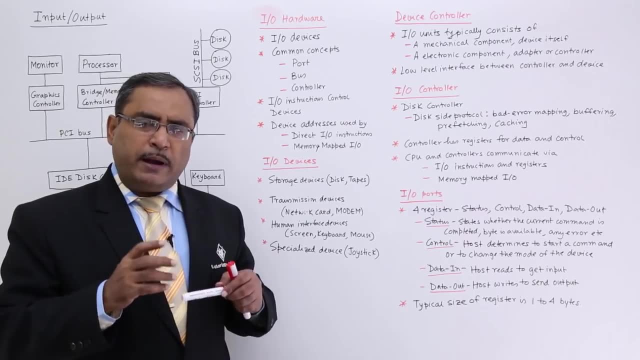 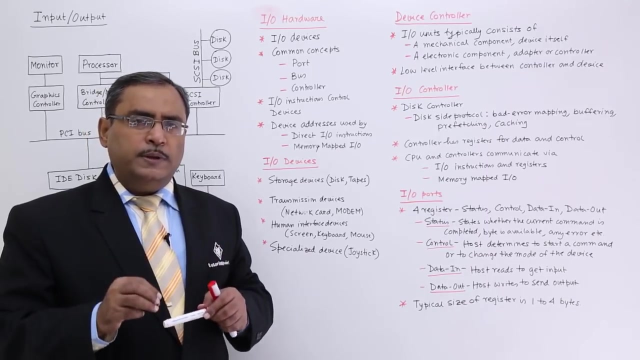 IO. In case of IOMapped IO, there will be some dedicated instructions are there, with the help of which the communication will be established. This dedicated instructions might be in or out, with the help of which we can do the communication with the IO devices, and there will be some. 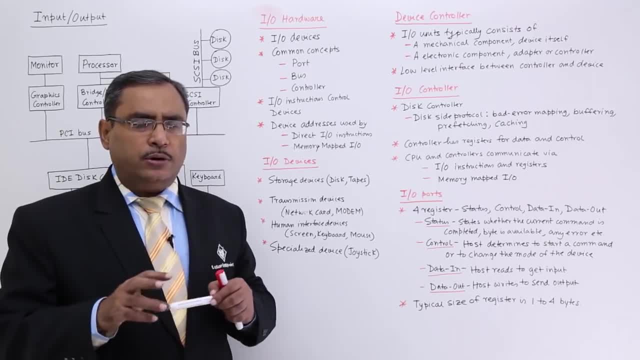 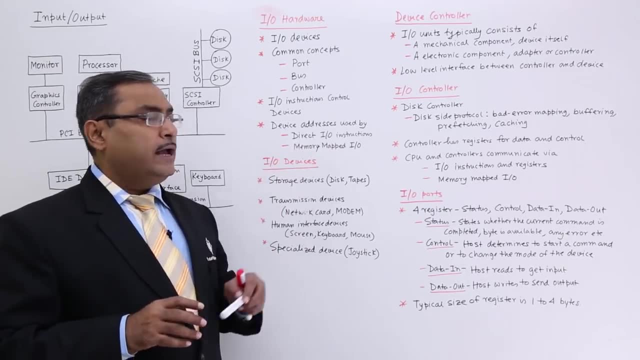 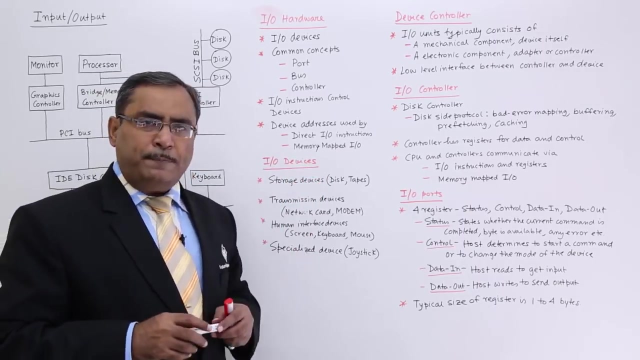 dedicated IO control signals- Say IO read or IO write- will be used to establish the communication with the IO devices. So that is known as direct IO instructions. So in this case we will be having dedicated instructions and dedicated control signals In case of memory mapped IO. all those instructions. 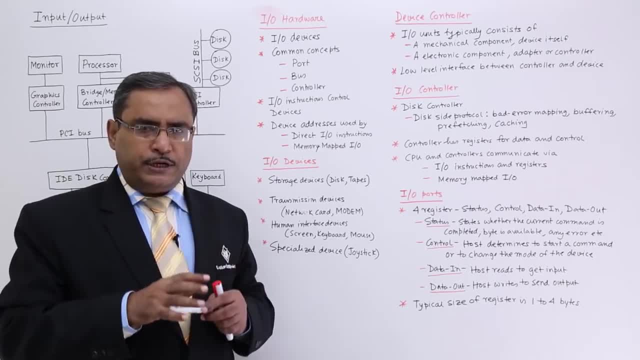 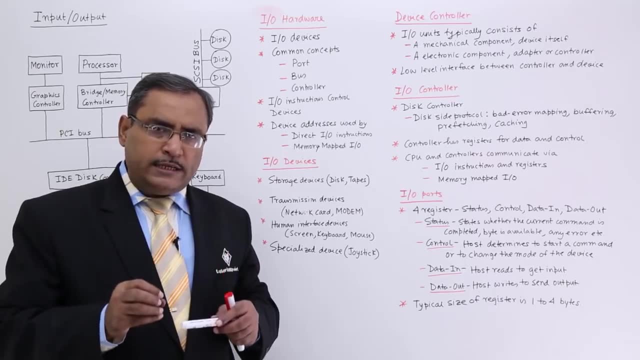 which are being used for the memory read or memory write operations. all the control signals which will be used for the memory read or memory write operations will be utilized for the IO read and IO write operations. So, in case of memory mapped IO, all those instructions. 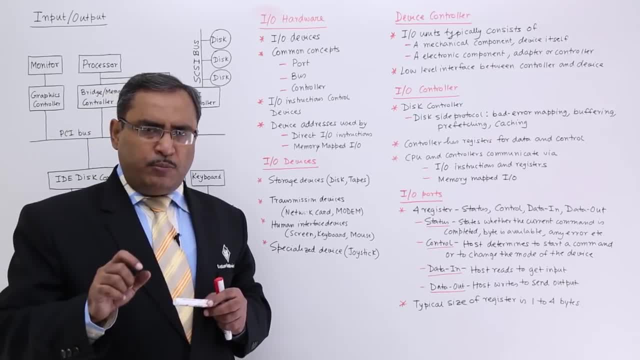 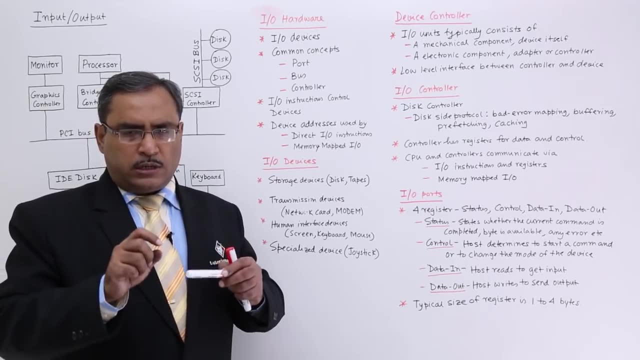 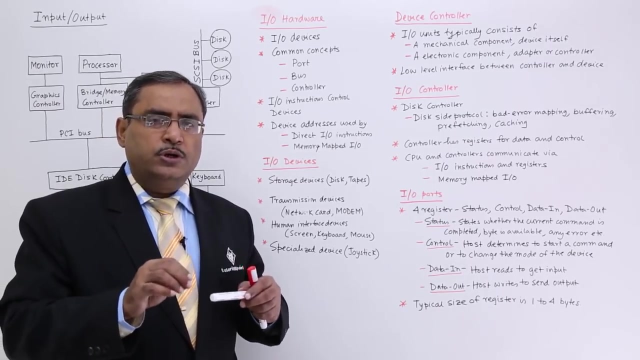 will be utilized for the memory read and IO write operations. So that means here each and every memory location. some of the memory locations will be replaced by the IO devices. and what about the control signals? what are the instructions we were supposed to used to access those memory locations? Now they will be used to do the communication with. 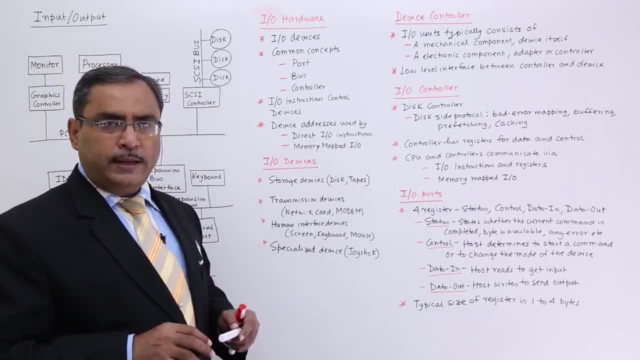 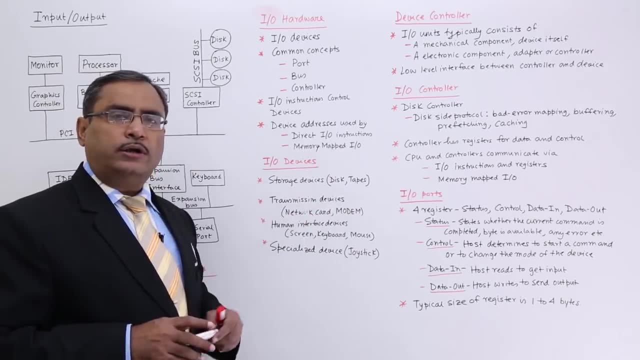 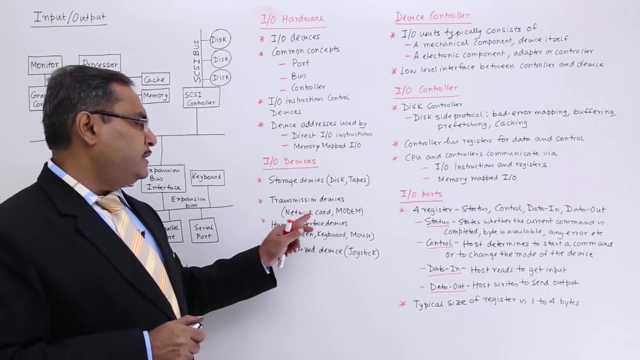 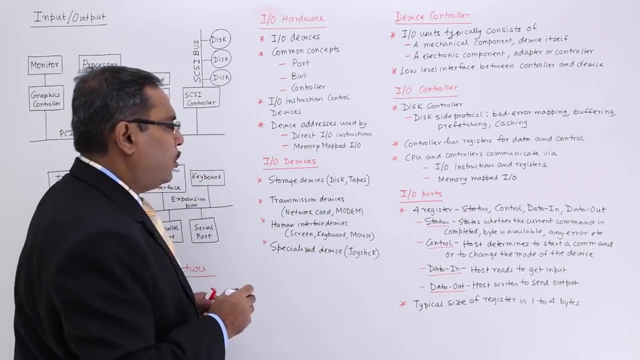 the IO devices, and that is why it is called memory mapped IO. This IO devices can be categorized mainly into four heads. One is the storage devices or tapes, and all these storage devices are of the type block oriented device transmission devices like your network card modem. so it will be so, all these ah transmission devices. 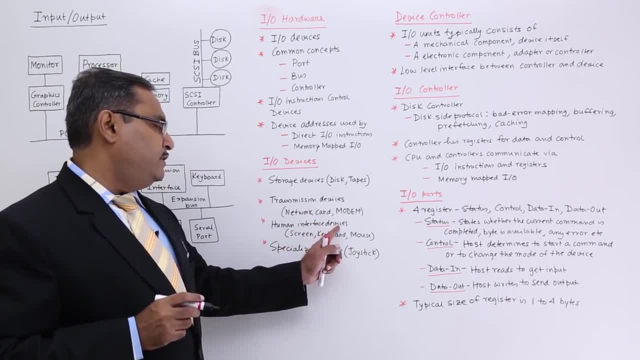 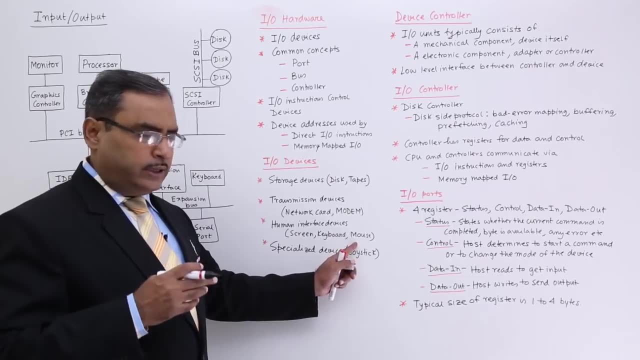 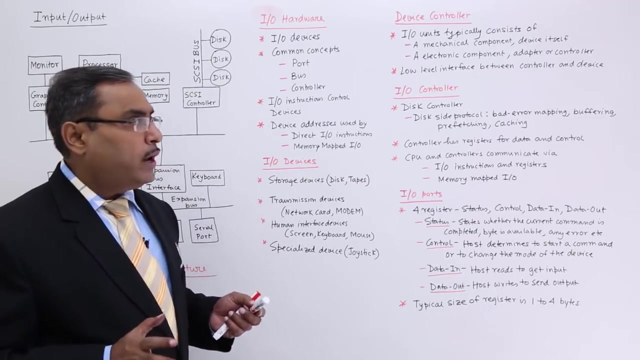 are like network card or modem, say human interface devices like your screen, the output device. there is a keyboard that is input device, and the mouse, that is also the input device, and specialized devices like joystick. so in this way this i o devices can get categorize mainly. 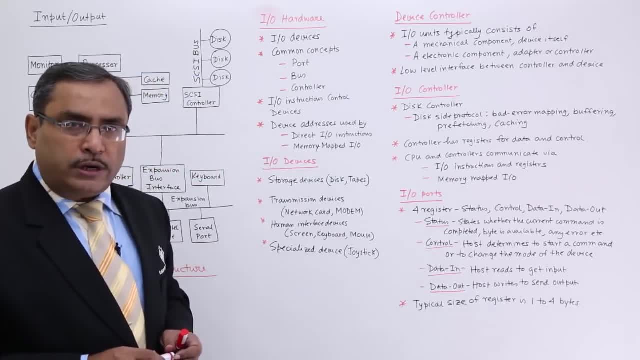 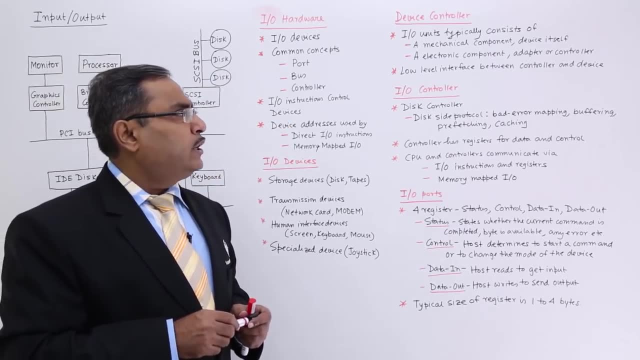 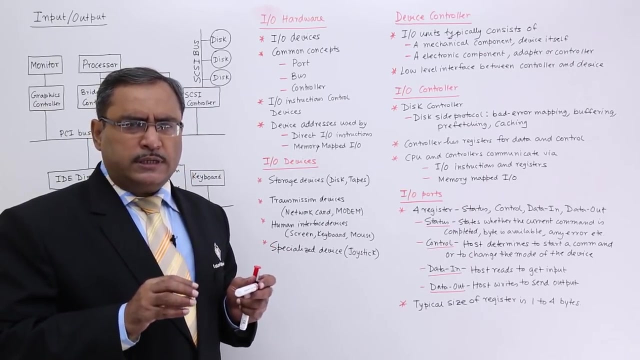 into broad categories. we are having the device controller, device controller. i have mentioned 2 features. 1 is the i o units. typically consists of a mechanical component, that is a device itself, say one storage device, hard disk. there are so many mechanical components are there residing within the hard disk and they will play the wider role for the read and write. 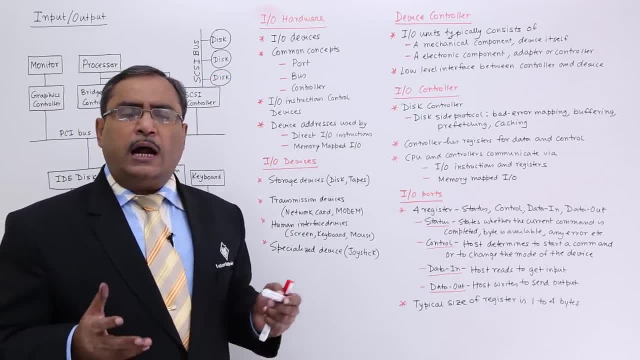 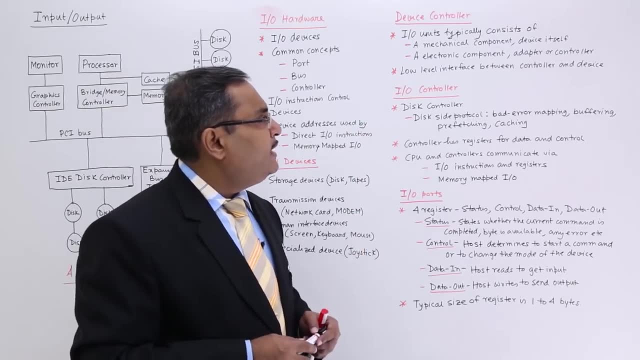 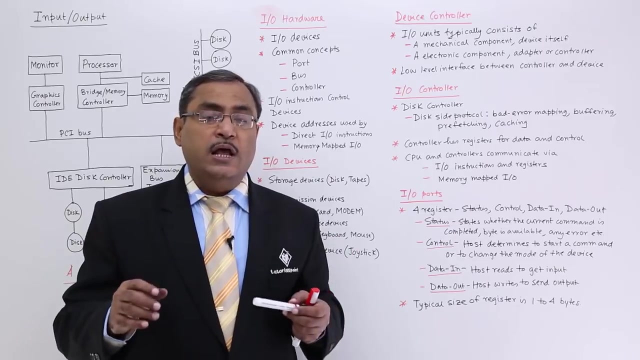 operations. another one is a electronic component- it might be an adapter or a controller which will establish a communication between the system and the i? o device and low level interface between controller and the device. so controller and the device will be the low level interface. low level interface means the controller will issue certain control commands which operating 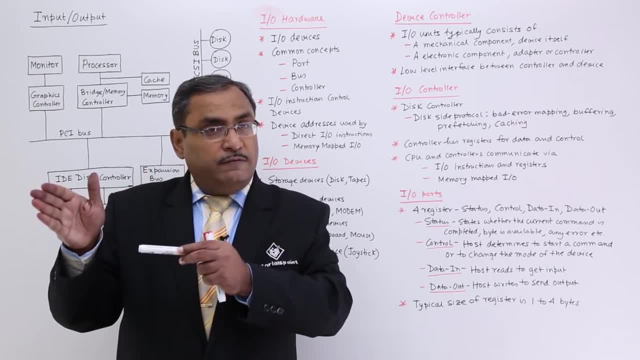 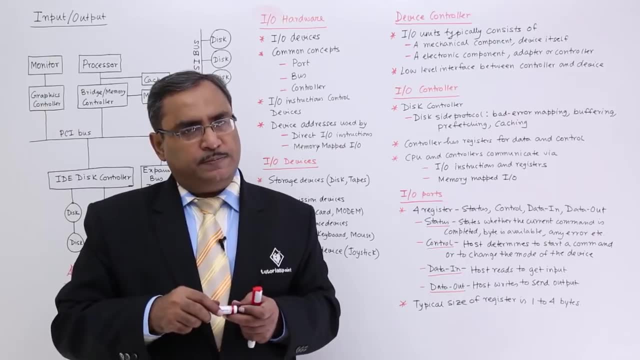 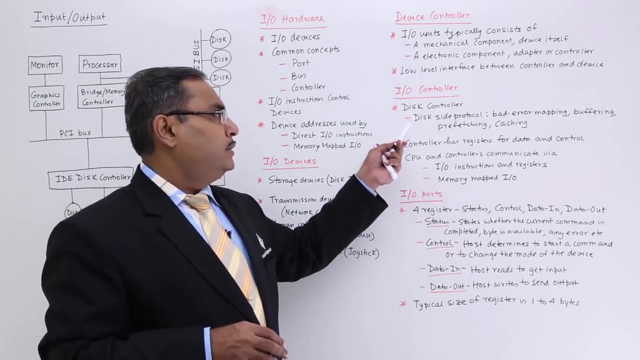 system may not interpret, but those that very particular device will be knowing what is the meaning of those commands. so only controller can issue those commands to the respective devices. so that is the low level interface between the controller and the device, where having the i o controller can be categorized into three heads, whatever i have mentioned. 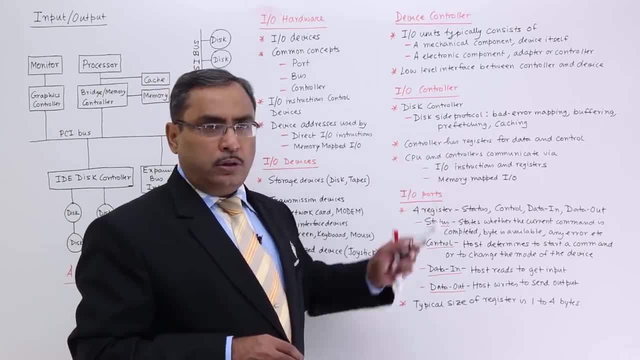 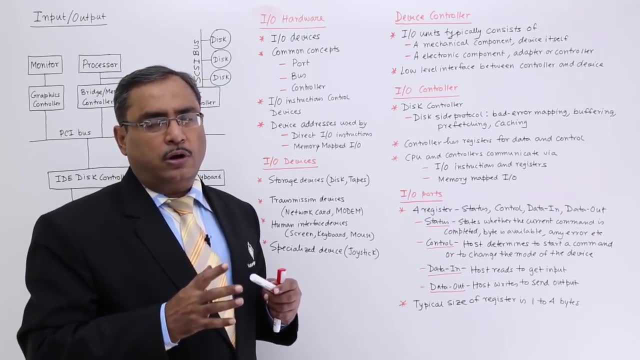 here one is a disc controller, so that is a disc site protocol. so that means this disc controller can detect whether the data transmission has been completed or not, can detect errors, can do the buffering, can do the prefetching, can do the buffering, can do the prefetching. 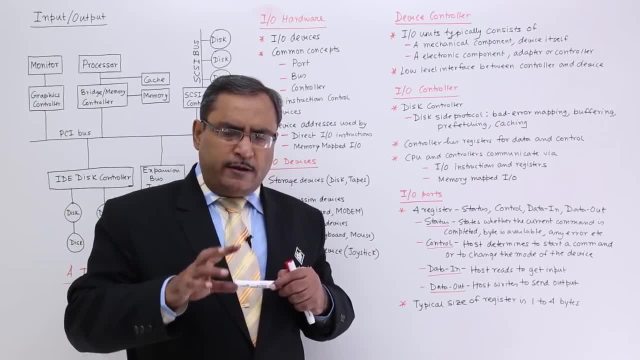 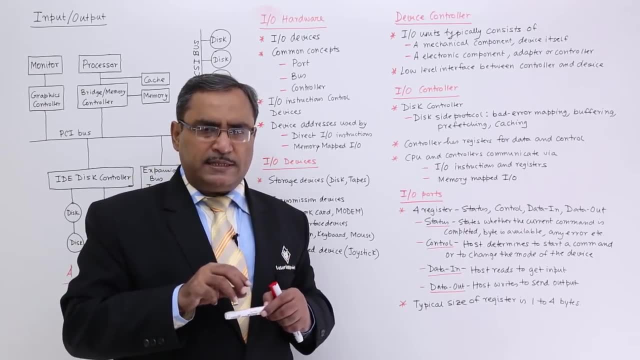 if i know that next data is going to be read from the very track and sector, from that very block, so i can prefetch that amount of data within the buffer space so that whenever it will be require, it can get supplied. so thus why this sight protocol can detect whether 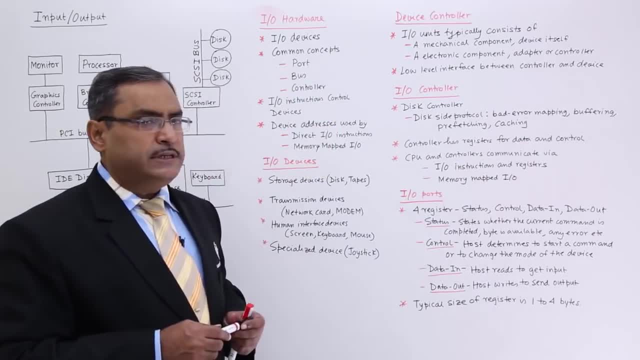 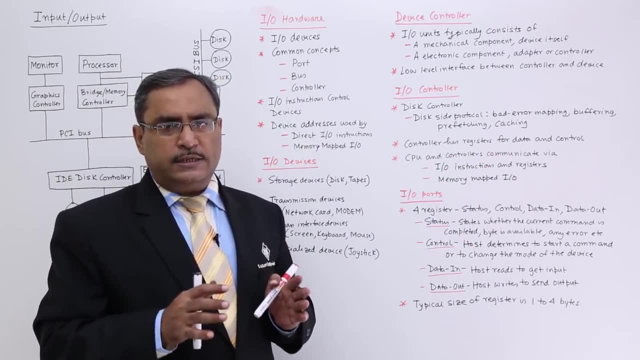 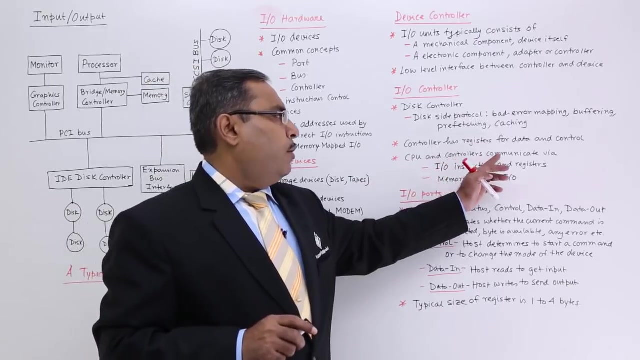 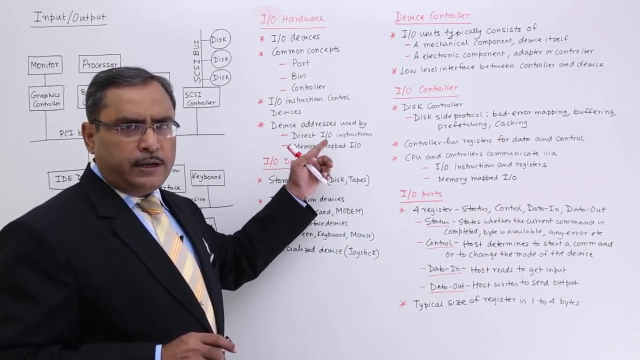 any error has occurred or not. can do the buffering, can do the prefetching and caching. controller has registers for data and control, so controller itself will have some registers dedicated to hold some data, to have some control words. CPU and controllers communicate via IO instructions and registers or memory mapped IO, whatever. we have discussed little bit here. so IO instructions and registers. 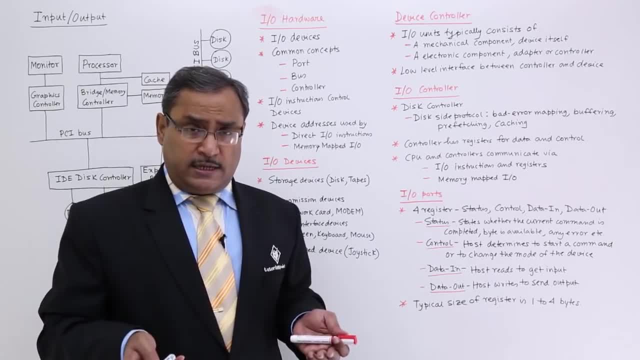 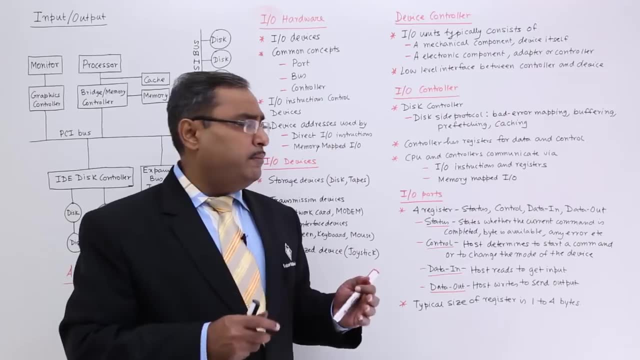 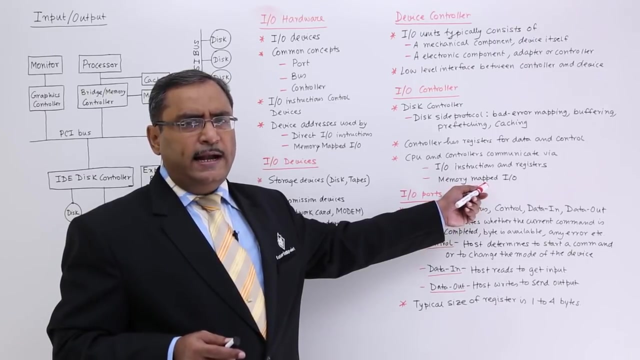 we know I told you that to such instructions are in instruction and out instruction. in case of memory mapped IO, the instructions can be memory read or memory write. so now we are having this IO ports memory map. some instructions like be your LDA, STA store accumulator, load accumulator type. 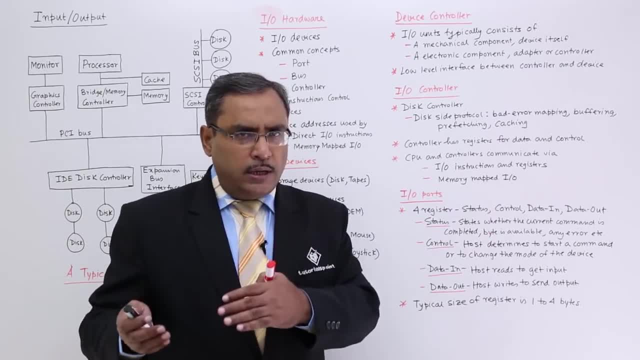 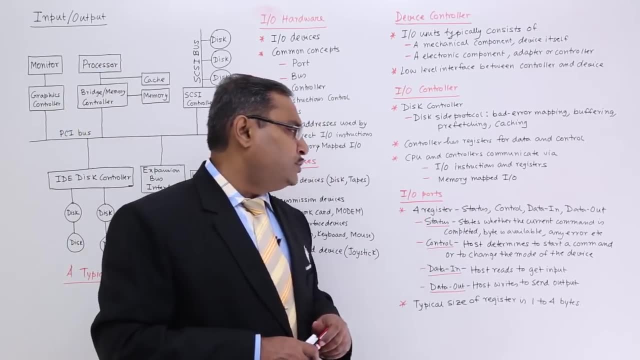 of instructions might be there. so using the same instruction, I can do the read write from the memory. using the same instruction, here I will be doing the read write from the IO devices. so IO ports merely is having four kinds of registers: one is the status, next one is the control, next one is